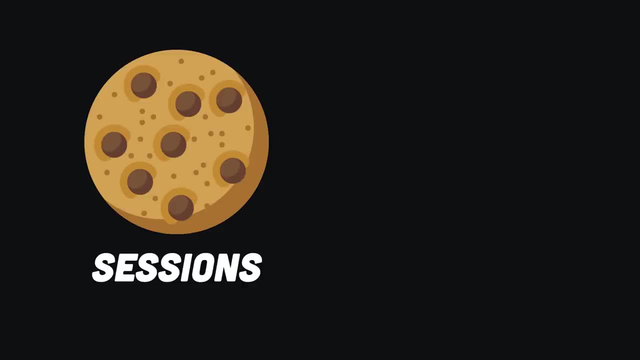 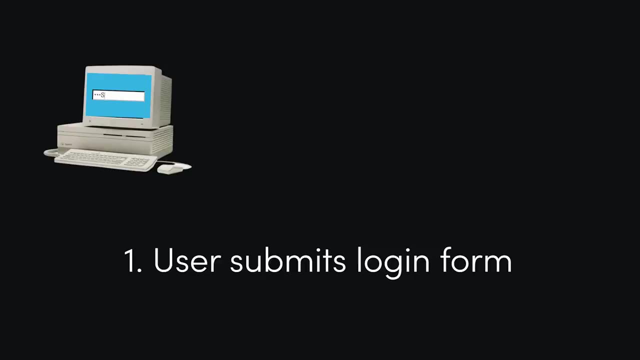 User authentication. There are two main ways to get the job done: Sessions and tokens. The traditional approach on the web is cookie-based server-side sessions. The process begins with a user filling out their username and password and then submitting it to a server, which then 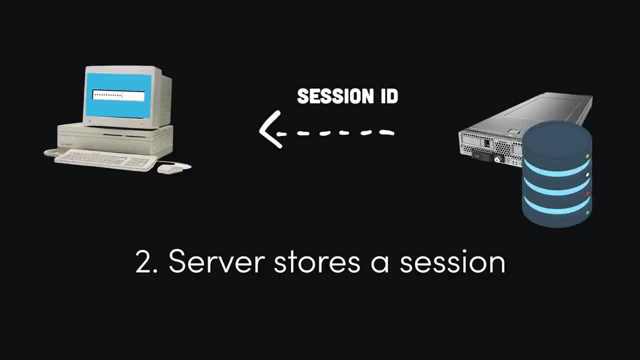 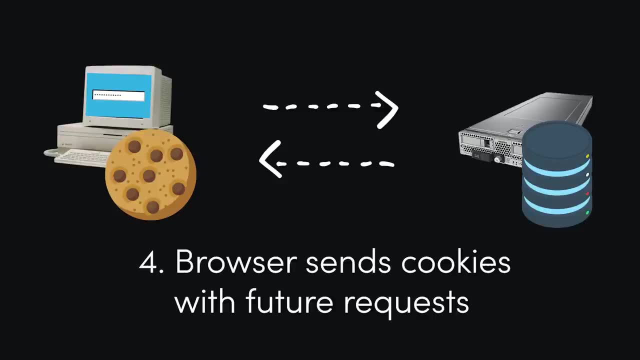 validates it, creates a session in the database, then responds with a session ID. The session ID will be saved in the browser's cookie jar, which is a place in the browser to save key value pairs that will be sent back to the server on each subsequent request. It can then respond back. 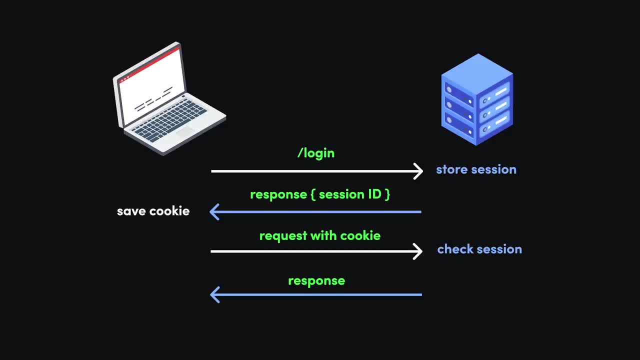 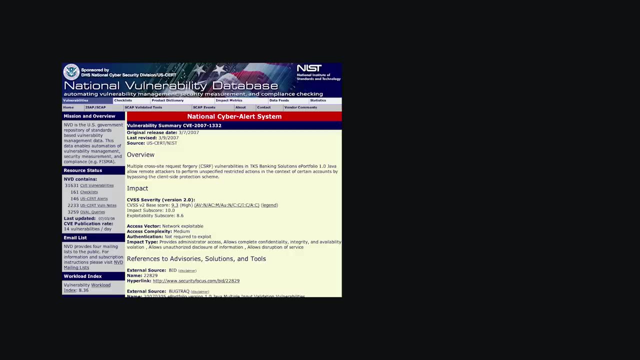 with content designed for the currently logged-in user. In other words, we have a stateful session between the front-end client and back-end server. This approach works great, but there are some drawbacks. It can be vulnerable to an attack known as cross-site request forgery, where the attacker 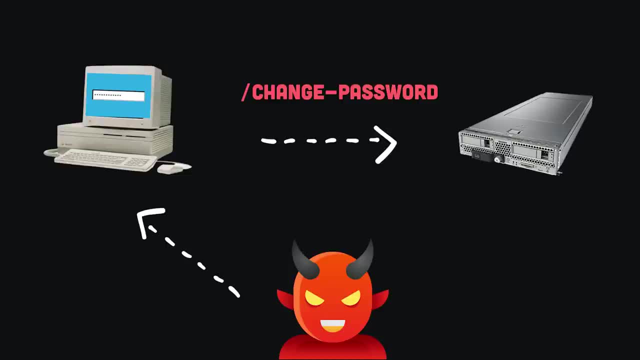 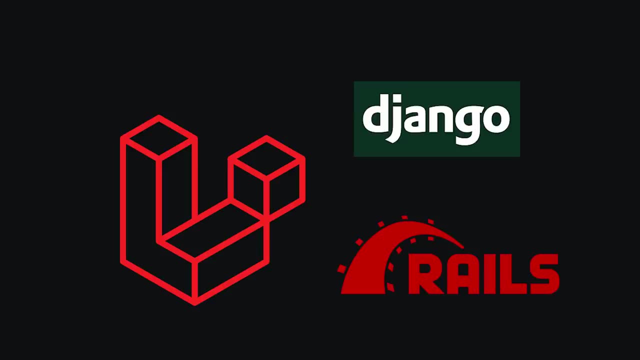 points the user to a site they're logged into to perform actions they didn't intend to like submitting a payment or changing their password. although the risk is very low, especially if you use a modern framework to implement your code, The bigger problem is that you'll need to store. 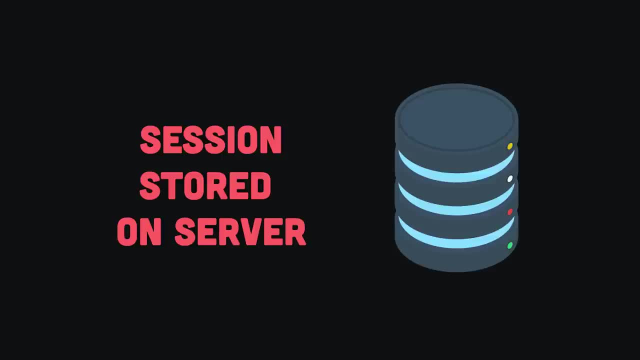 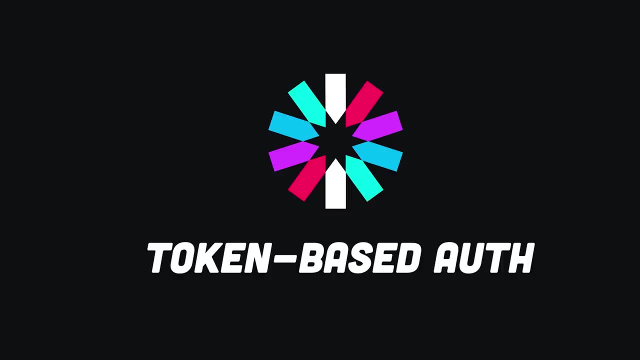 the session ID in a database or keep it in memory on the server. Because most of today's cloud applications are scaled horizontally, this can be a huge bottleneck in production, And that brings us to token-based authentication, which solves this problem but introduces its own set of challenges. The process begins the same with the client. 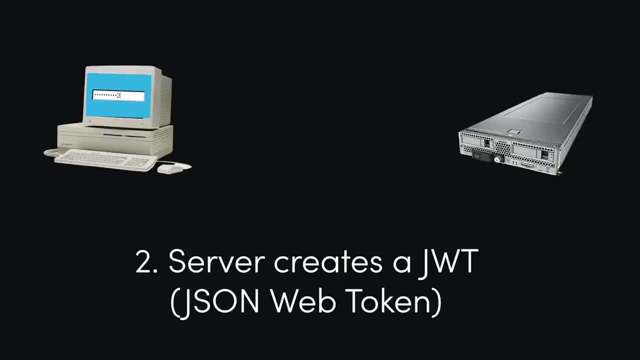 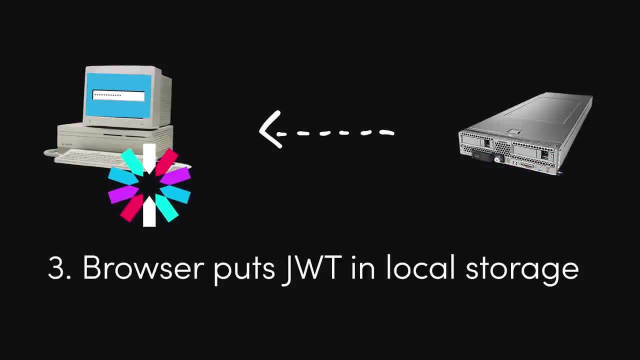 sending its login details to the server. Instead of storing a session ID, it generates a JSON web token. The JWT is created with a private key on the server. then it's sent back to the browser, where it's normally kept in local storage. On future requests, the JWT will be added to the 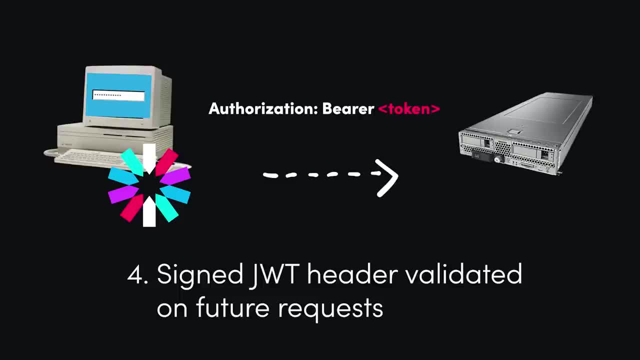 authorization header prefixed by bearer. The server then only needs to validate the signature. There's no need for a database lookup somewhere else in the infrastructure, and that's way more efficient. when dealing with a distributed system. in the cloud, However, tokens can still be hijacked by an attacker, and they can also be 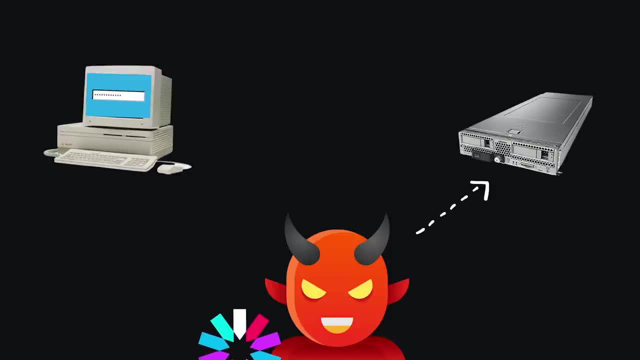 difficult to invalidate and they can't be used to authenticate a user in the background on the server. Here's the most important thing to understand. With a session, the authentication state is handled on the server, while tokens are managed on the client. This has been user.